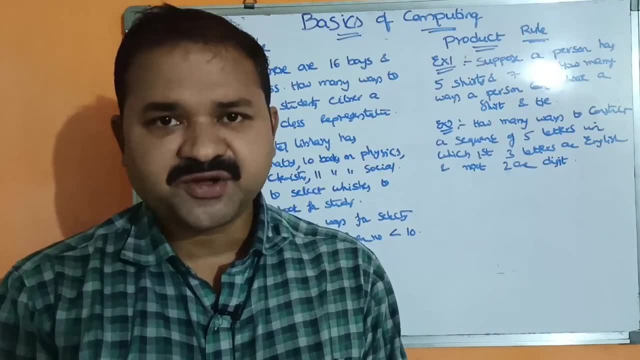 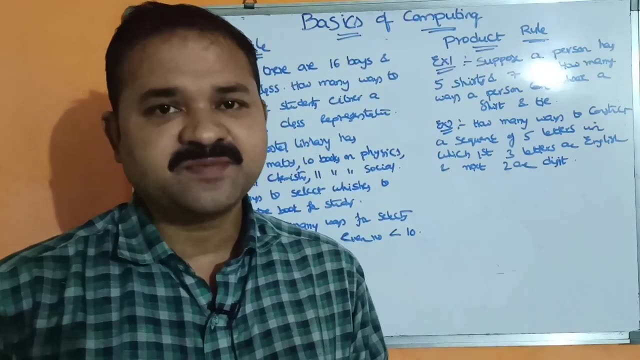 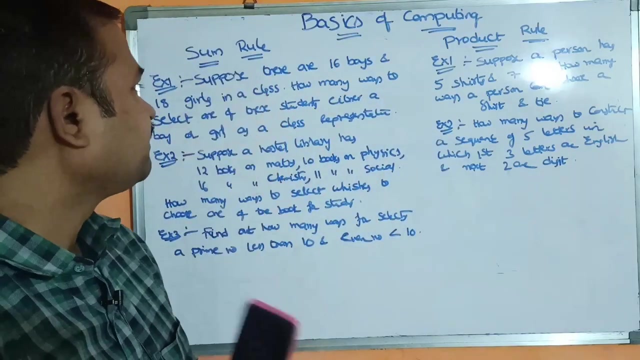 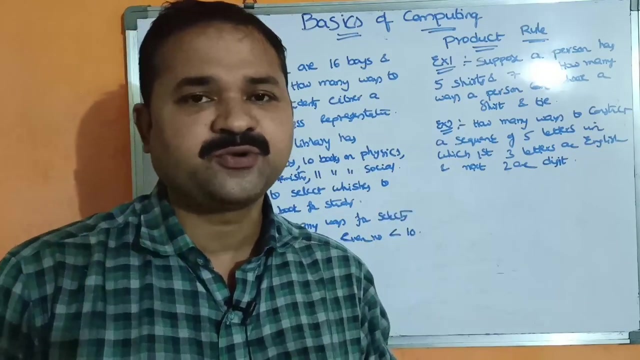 In this video we are going to discuss about basics of computing in combinatorics, discrete mathematical structures. Mainly, we can perform computing in two ways. The first way is sum rule. The second way is product rule. First let's see what is sum rule and product rule. 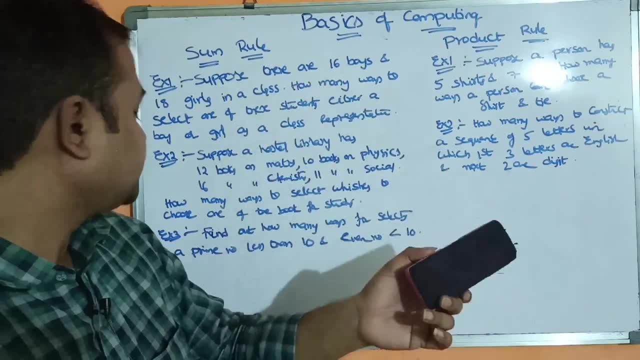 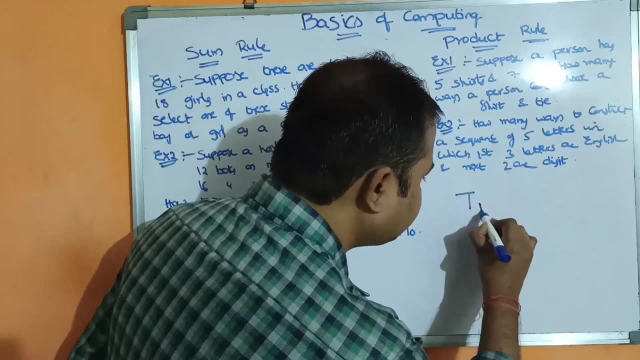 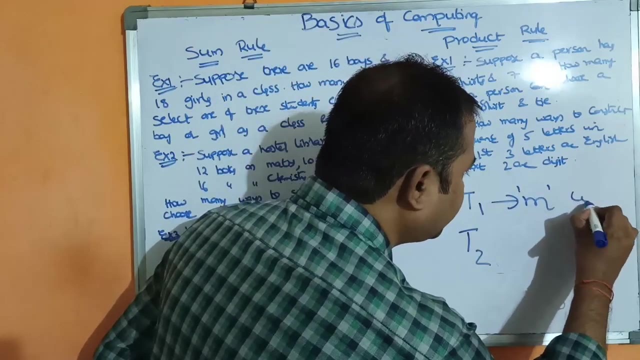 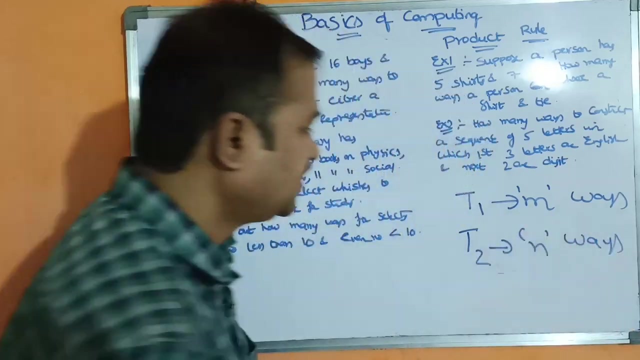 And then we are going to solve three examples on sum rule and two examples on product rule. Let we have two tasks, such as t1 and t2.. Let task t1 can be performed in m ways. Let task t2 can be performed in n ways. Here, sum rule means out of the two tasks. 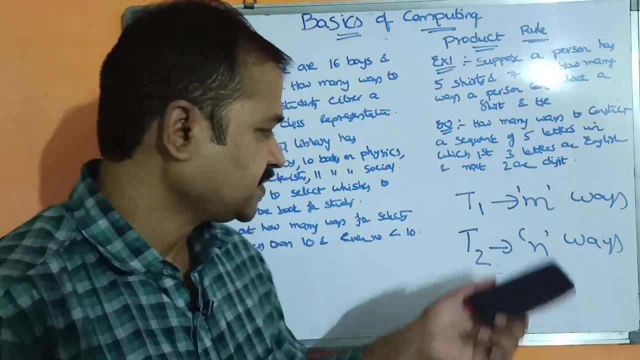 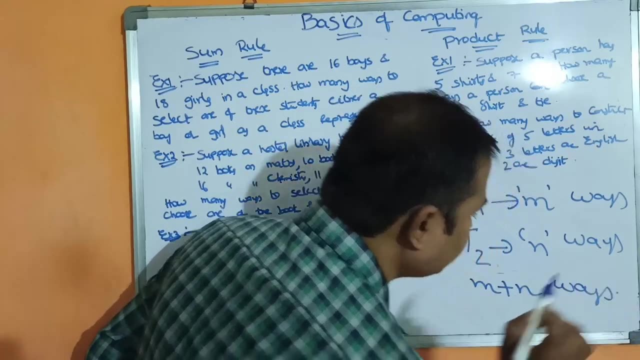 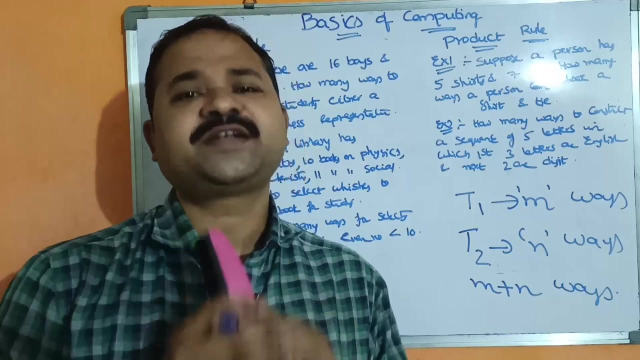 we can perform one task, Only one task. Sum rule means we can perform only one task in m plus n ways. So sum rule means it is not possible to perform the two tasks. So we have to perform only one task between t1 and t2 and it is some operation. So we can perform in m plus n ways. 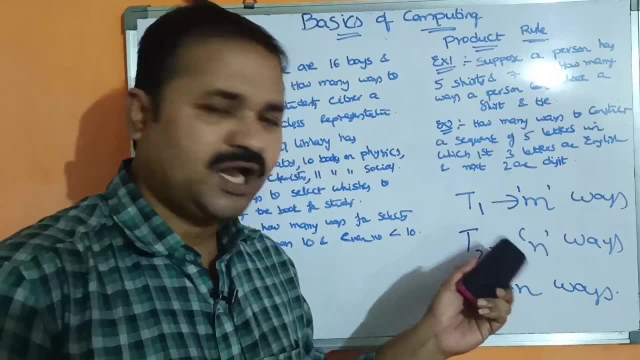 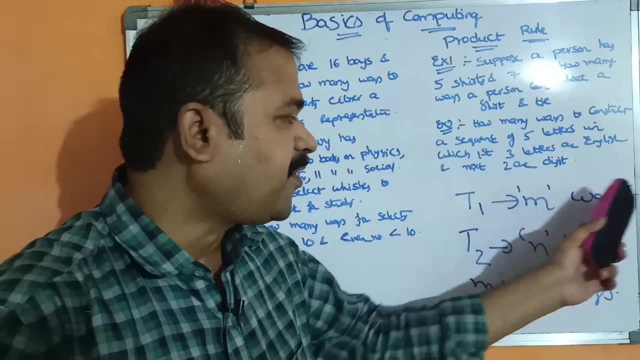 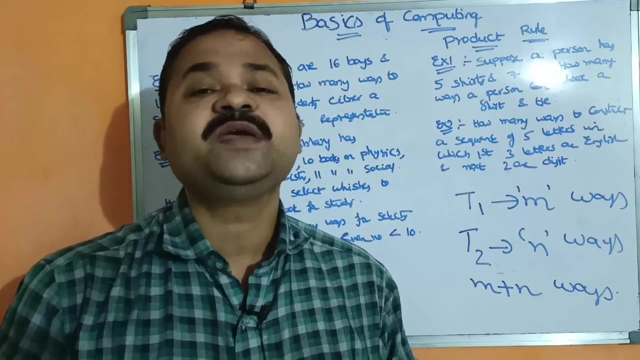 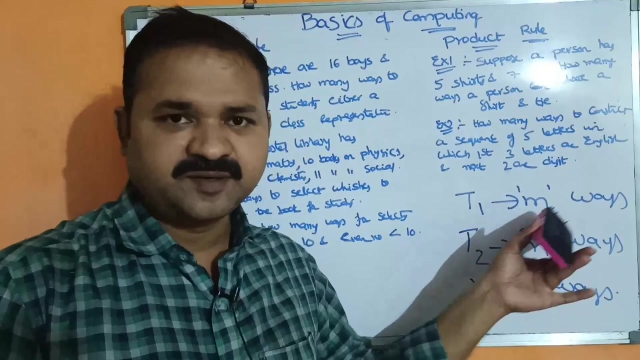 Now let us see what is product rule Here also, let we have two tasks, such as t1 and t2.. Let task t1 can be performed in m ways. Let task t2 can be performed in n ways. Product rule means we have to perform both the tasks, So task by task. So first t1 will be performed and then 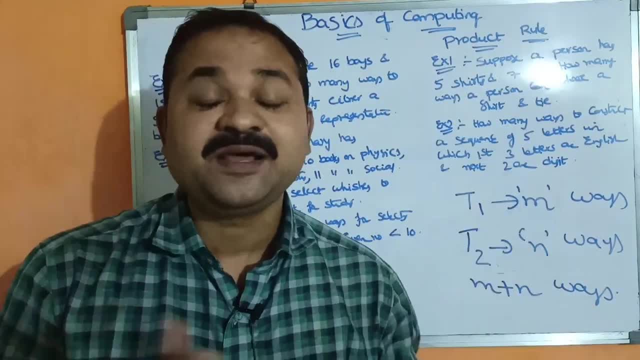 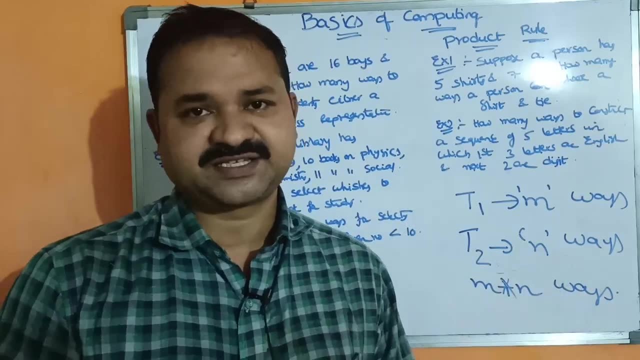 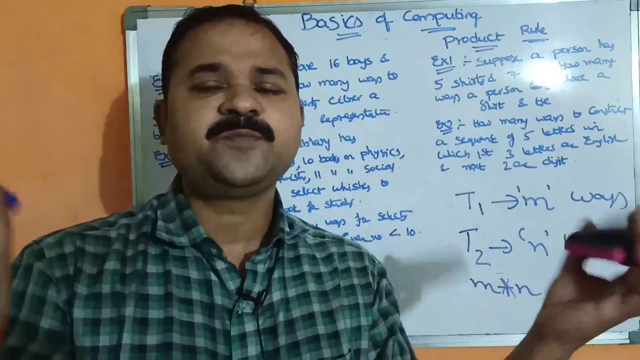 t2 will be performed. So product means multiplication operation. So we can perform both the tasks in m into n ways In m into n ways. So sum rule means we can perform both the tasks in m plus n ways. Out of all the tasks we can perform only one task. Product rule means we can perform. 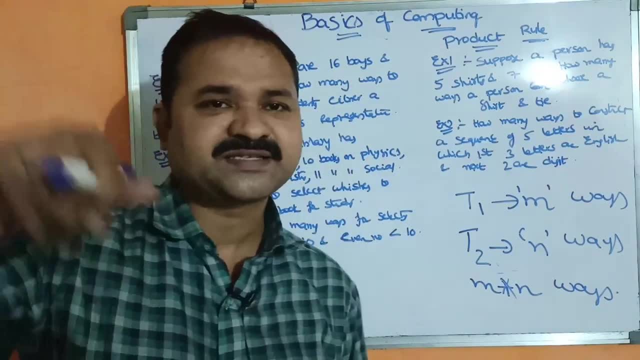 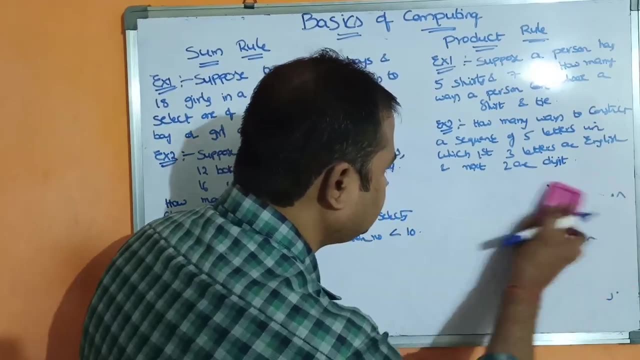 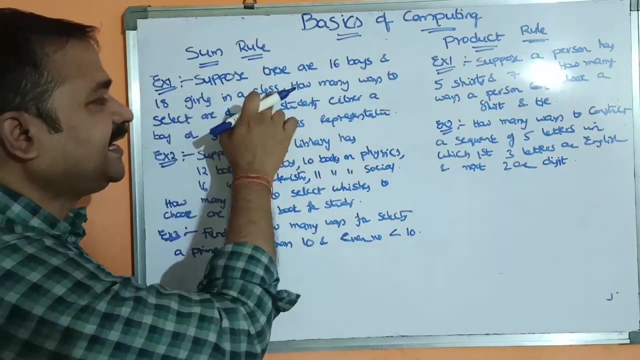 both the tasks one by one. So sum rule means plus operation, Product rule means multiplication operation. Now let us see examples on sum rule. Let us see the first example. Suppose there are 16 boys and 18 girls in a class. How many ways to select one of these students? 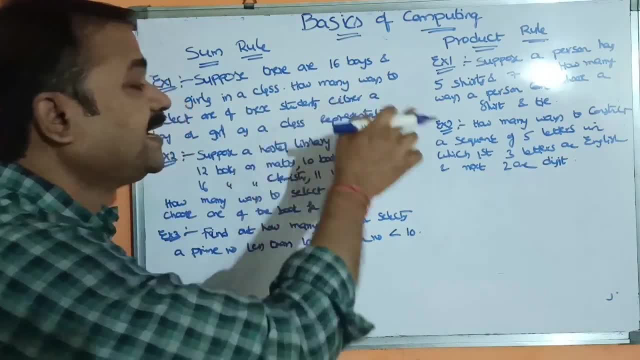 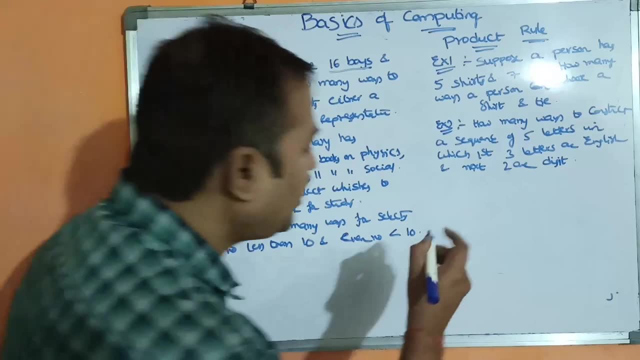 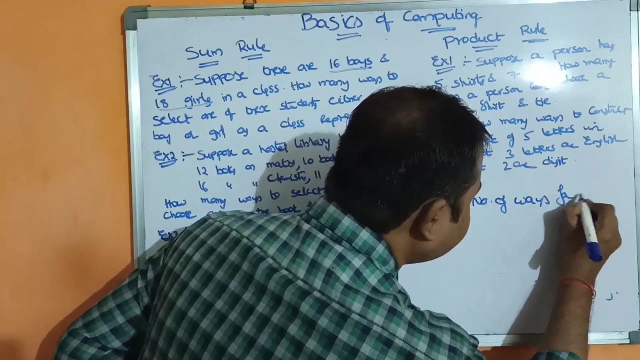 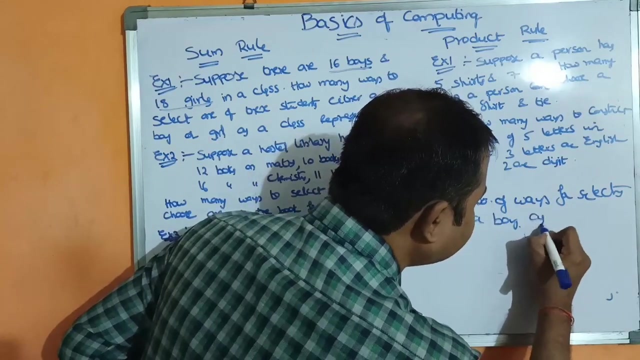 Either a boy or girl as a class representative. So here we are having 16 boys and 18 girls. So what is t1?? t1 means number of ways, number of ways for selecting, for selecting a boy as class representative, A boy as class representative. So that is t1.. So how many boys are there? 16.. 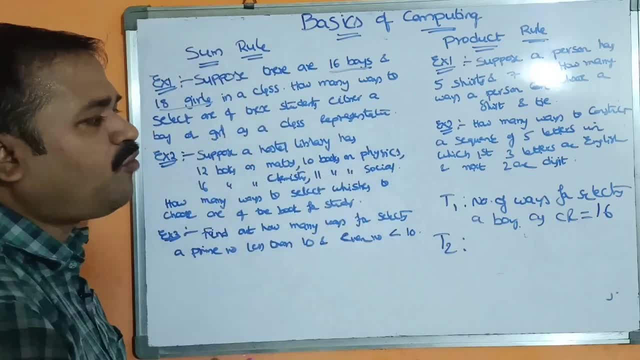 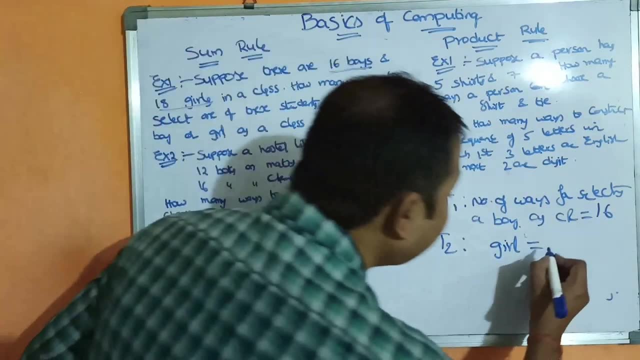 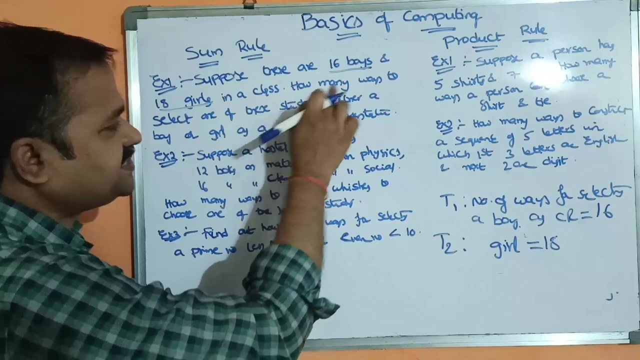 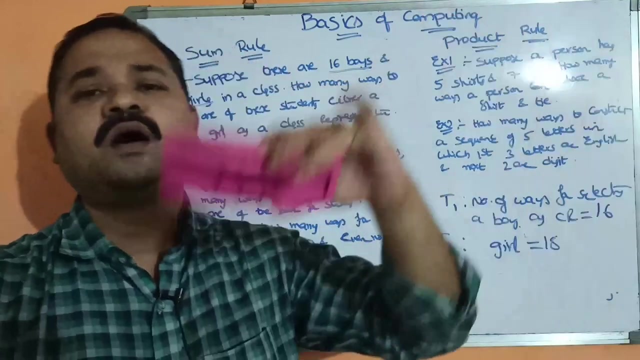 Next to t2 means number of ways for selecting a girl as a class representative. So how many girls are there? 18 girls. Next, let us see the problem: How many ways to select one of these students- Either a boy or girl- as a class teacher. So here we have to select either boy or girl. 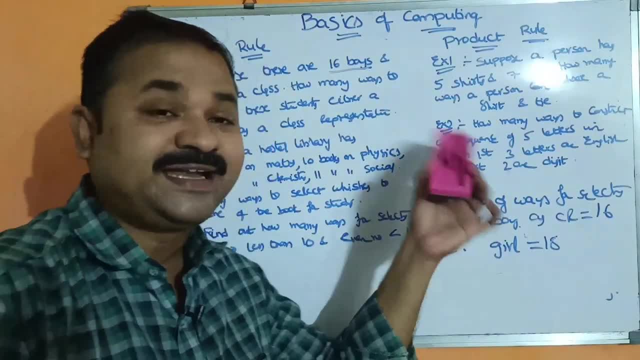 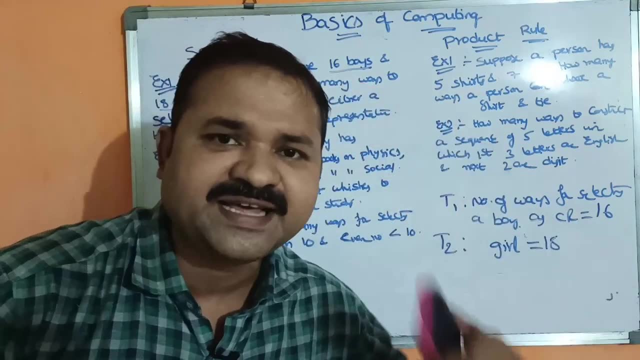 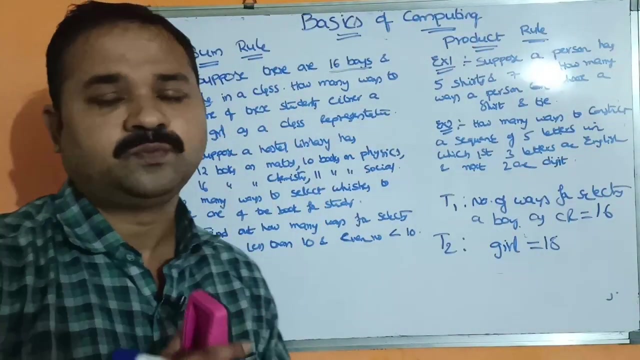 That means we can perform only one task, Either t1 or t2.. So that means which rule we have to apply now: Sum rule. Why? Because we have to select either a boy or a girl. That means we can perform either task t1 or task t2.. So we have to perform the sum rule. 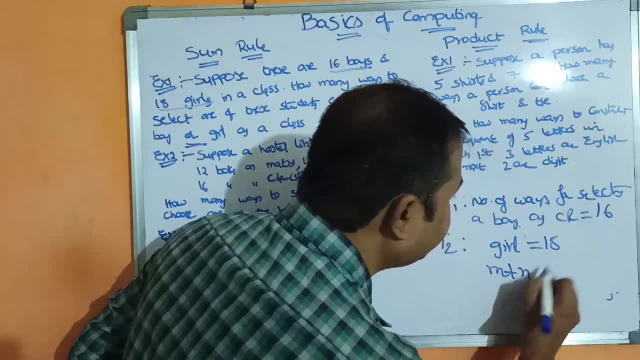 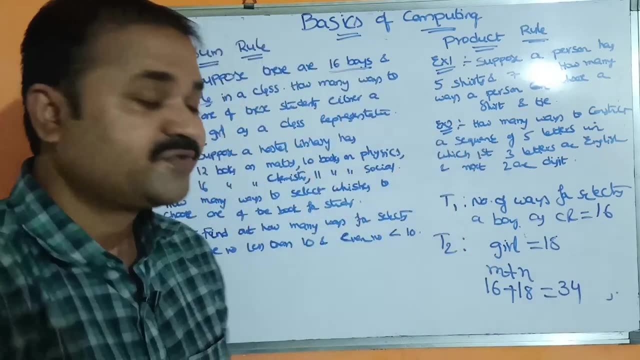 So what is sum rule? Simply add m plus n, So what is m 16.. What is n? 18.. So 16 plus 18 means 34.. So we have 34 ways, are there? So this is 16 ways, 18 ways. 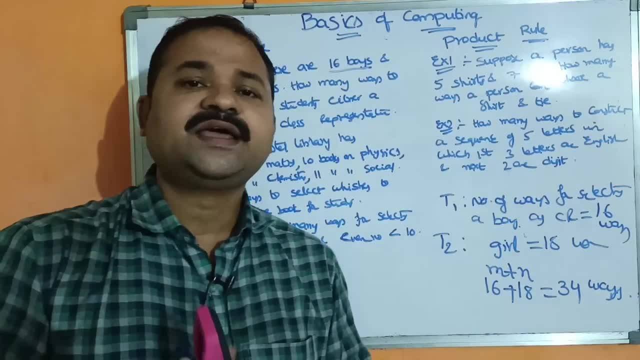 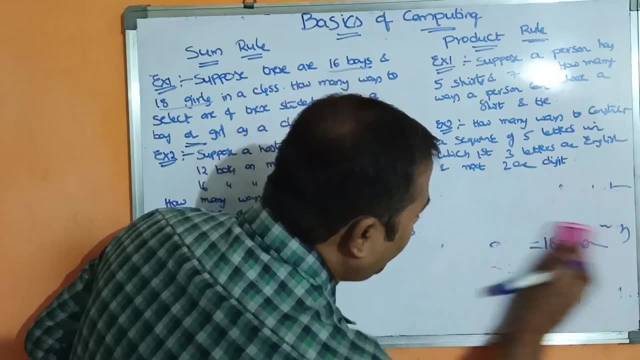 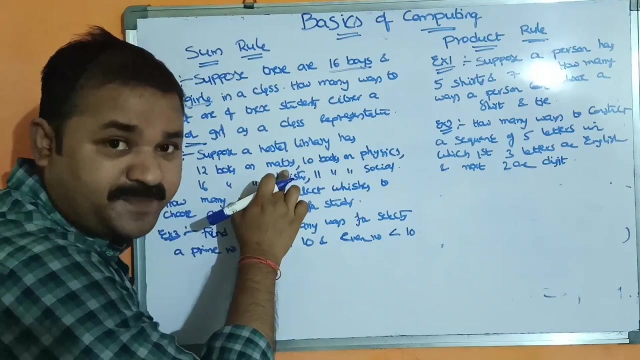 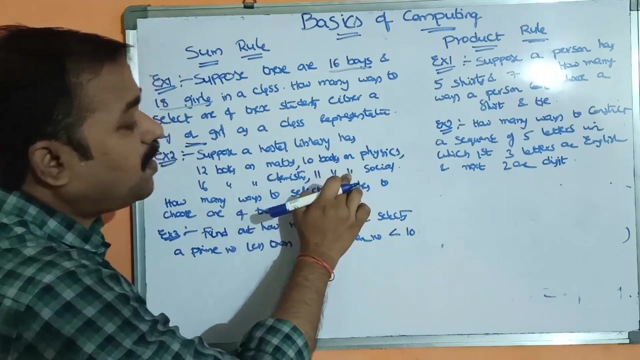 34 ways. So we have 34 ways are there in order to select either a boy or girl as class representative. Now let us see the second problem. Let us see the second problem. Suppose a hostel library has 12 books on mathematics, maths, 10 books on physics, 16 books on chemistry, 11 books on social. 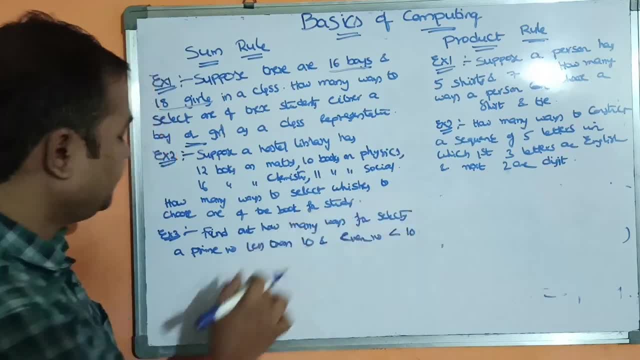 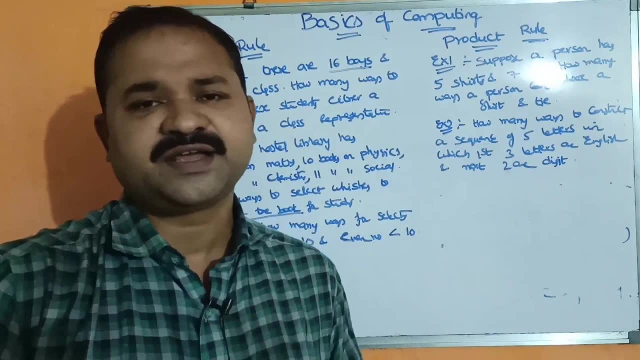 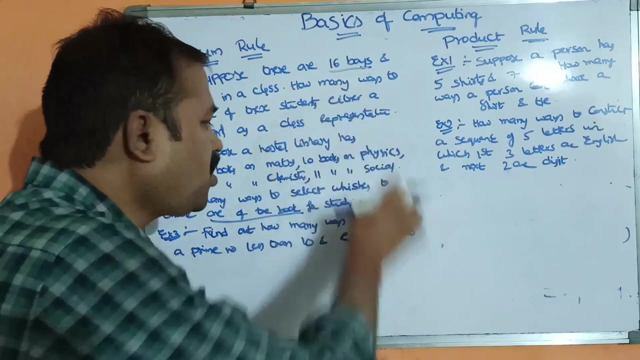 How many ways to select Wishes to choose one of the book for the study. So number of books are given Here. our target is: how many ways are there to select one book among all the books, So among all the books we have to. 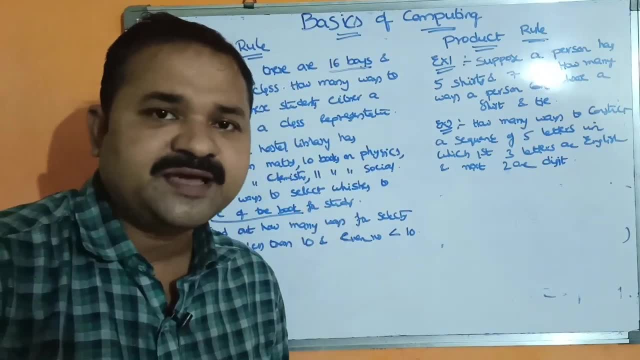 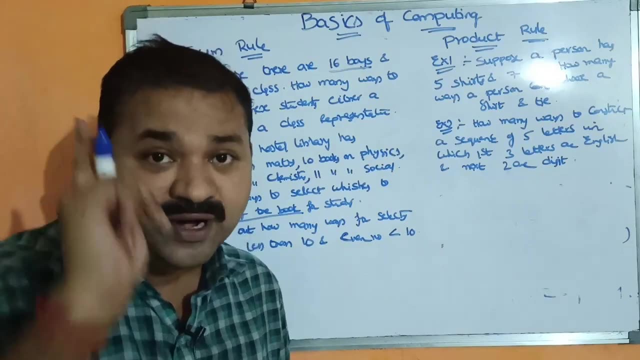 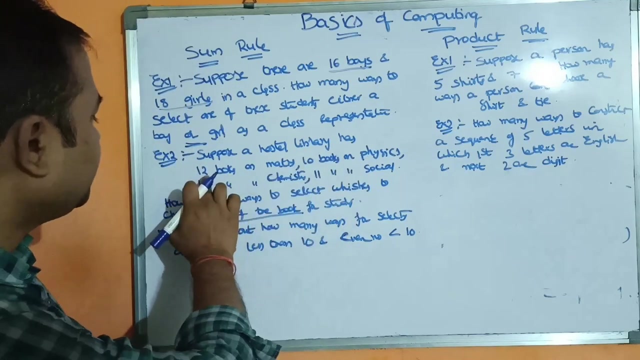 select only one book for study. It may be either mathematics book or physics book, or chemistry book or social book. So here we have to select. we have to perform only one task among all the tasks, So which will? we have to perform Some rule. So how many ways are there to select Mathematics book for study? 12 ways. Next, 10 books. 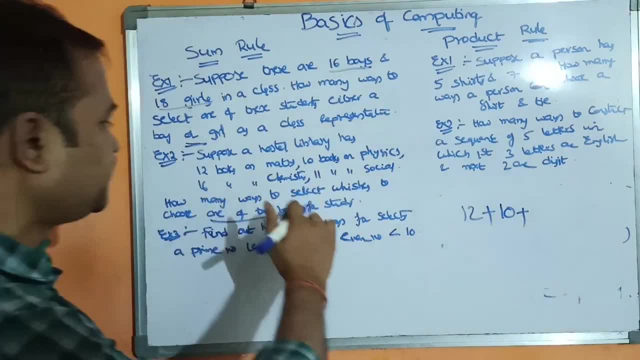 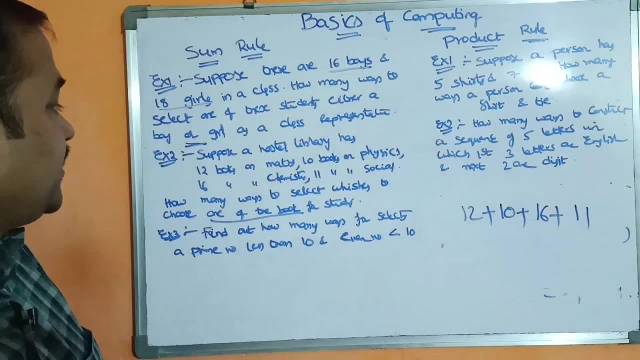 on physics. So 10 ways are there for studying the physics books, 16 ways are there for studying the chemistry. 11 books are there for studying the social. So 12,, 10,, 16,, 11.. So 12 plus 10 means 32.. 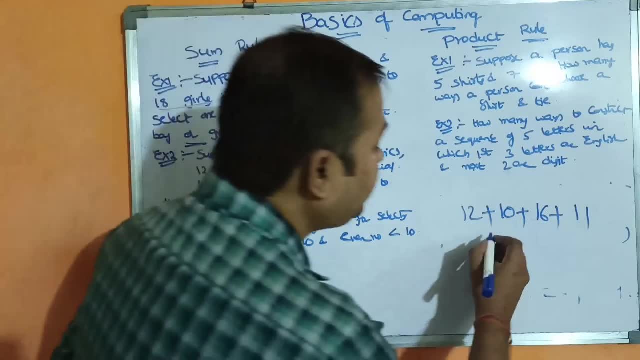 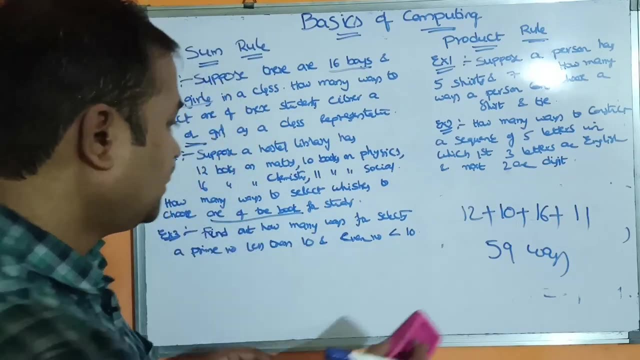 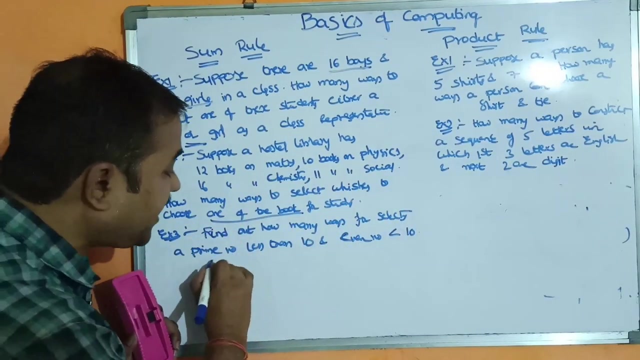 32 plus 16 means 48.. 48 plus 11 means 59. So, totally, there are 59 ways in order to choose one book for the study. Now let us see the next problem: Find out how many ways for selecting a prime number which is less than 10, and even 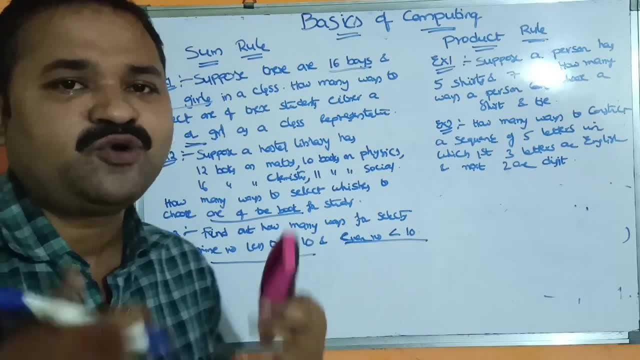 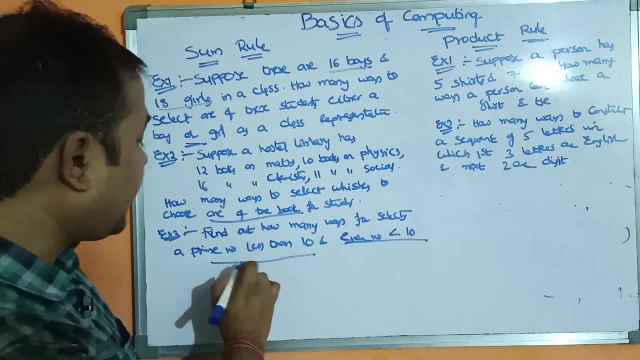 number which is less than 10.. So here we have to find out number of ways for selecting either: either for selecting either a prime number or a prime number which is less than 10, and it is- and an even number less than 10.. Okay, 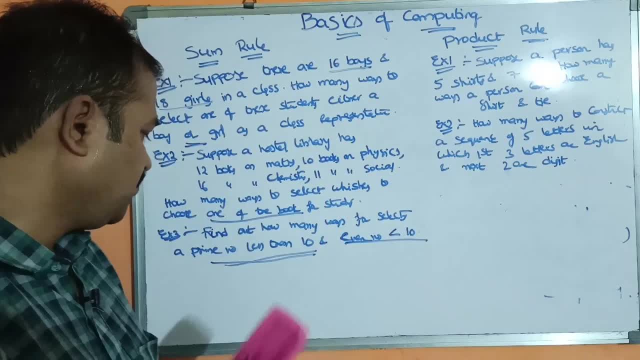 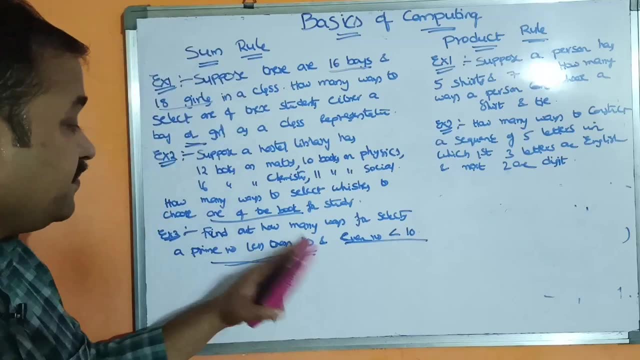 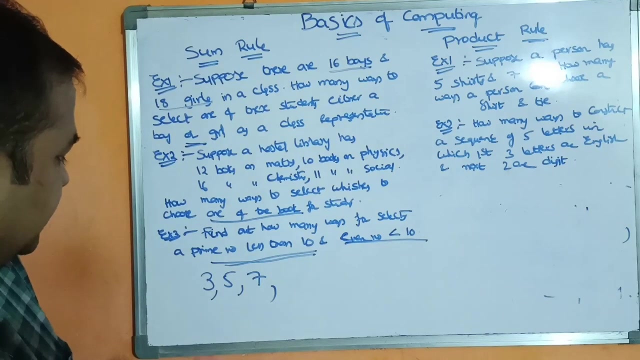 Here also we have to perform the sum rule. Why? Because we have to select either prime number or even number, So, which is less than 10.. So what are the prime numbers which are less than 10?? So 3,, 5, 7.. So 3,, 5, 7.. So 2 is also prime number. So 2,, 3,, 5,, 7.. But one: 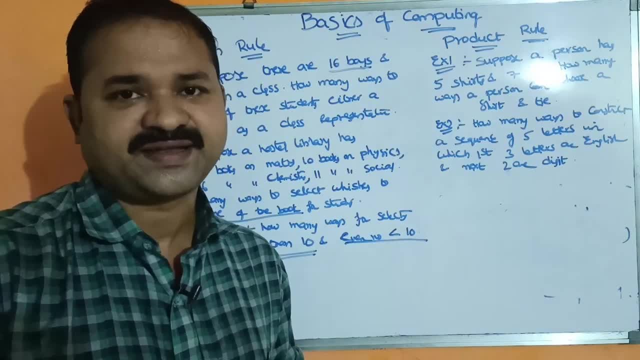 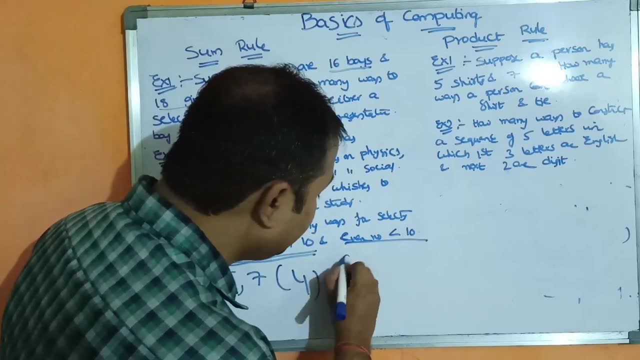 is not a prime number, because prime number means it should have two factors, but one has only one factor. So 2,, 3,, 5,, 7.. So there are four ways. Next, even numbers less than 10.. If we can consider 0 also, 0 is also even number. So 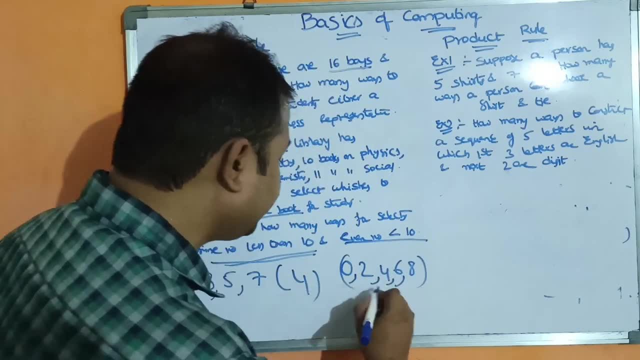 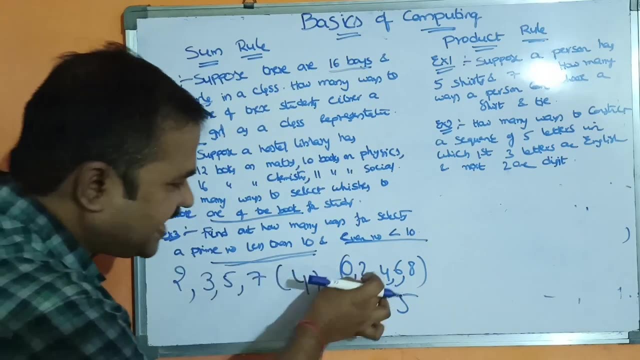 0,, 2,, 4,, 6, 8.. Okay, So how many ways are there? 1,, 2,, 3,, 4, 5.. So, 5 ways. Okay, But if we consider, 2,, 2 is present in this list as well as in this list. Okay, So we can ignore that. 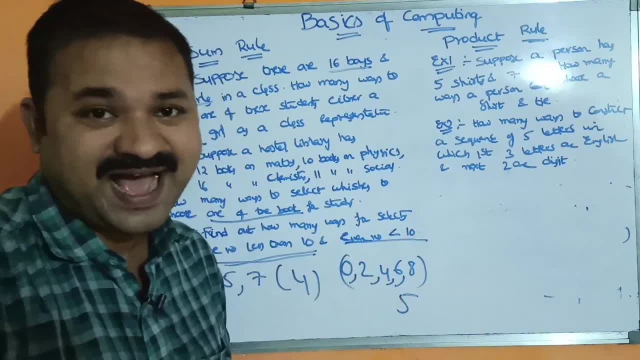 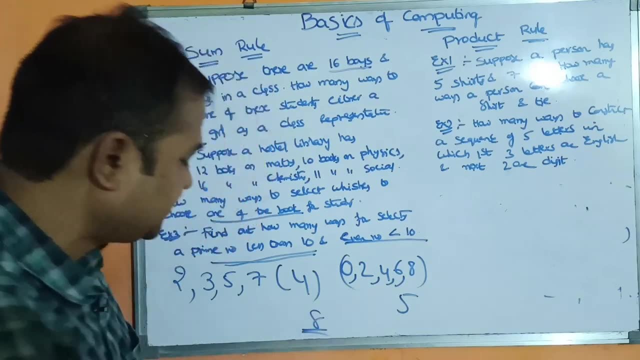 2. We have to consider only 1, 2. So 4 plus 5 means 9.. But we have to ignore 1, 2. Why? Because 2 is present in both the list. So 9 minus 1 means what? 8 ways? So there are. 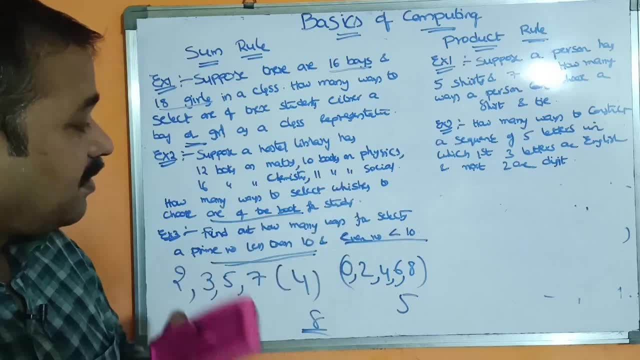 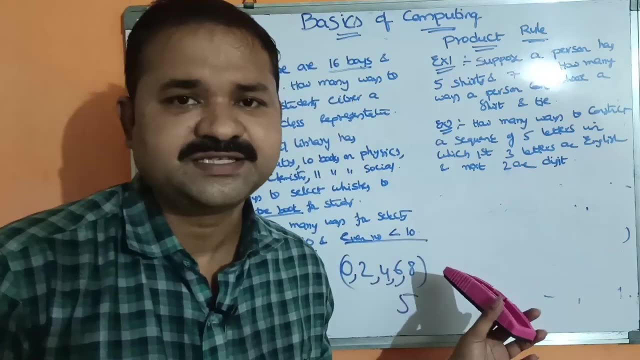 two ways in order to choose a prime number which is less than 10, or an even number which is less than 10.. Okay, Here it is less than 10.. So that's why here we are not considered 10.. Okay, Let us see the product rule. Product rule means we have to perform both the tasks. 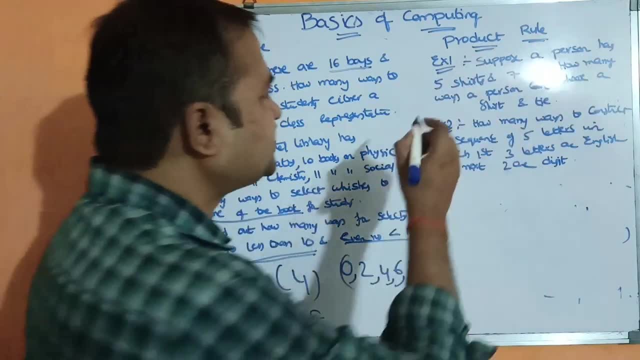 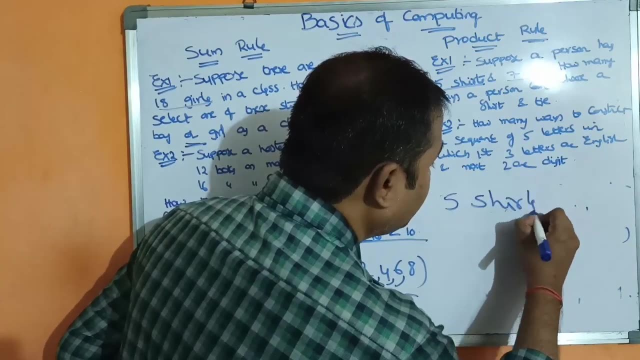 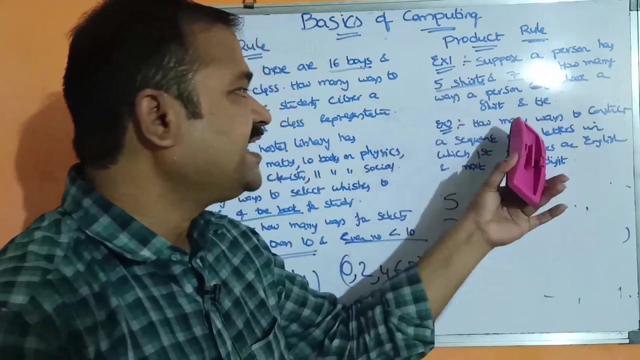 T1 as well as T2.. Suppose a person has 5 sheds and 7 ties. So person has how many sheds? 5 sheds, 5 sheds and 7 ties. how many ways a person can choose a shirt untied? so here the person has to wear both the things. 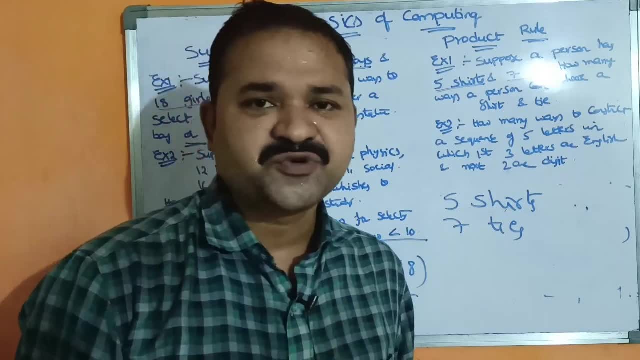 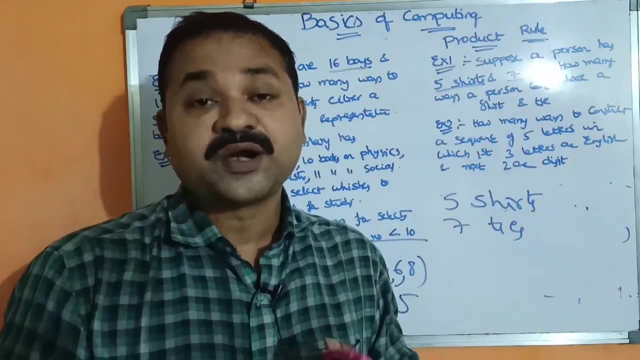 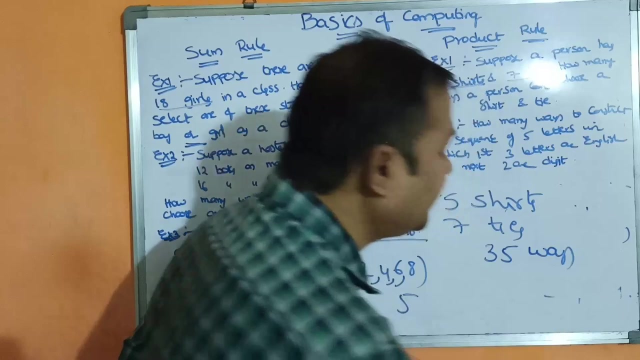 person has to wear shirt as well as person has to wear time, so we have to perform both the tasks. so both the tasks means we have to perform product rule. product rule means we have to perform the multiplication operation. so 5 into 7 means 35, so there are 35 ways in order to wear both shut as 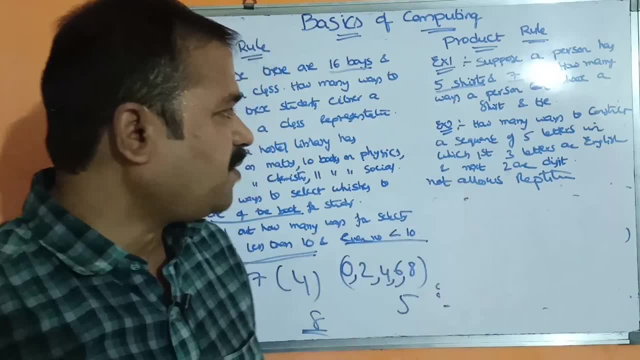 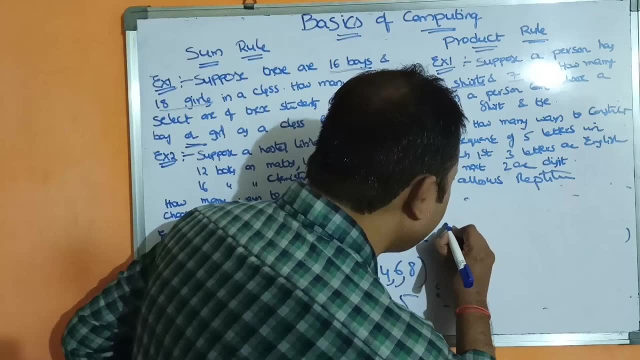 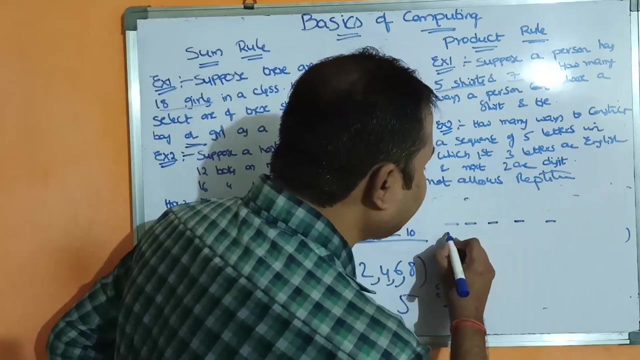 well, as time now, let us see the second problem: how many ways to construct a sequence of five letters? so here the sequence totally contains five letters: one, two, three, four, five, in which first two three letters are english, the first two three letters are english and the next two are: 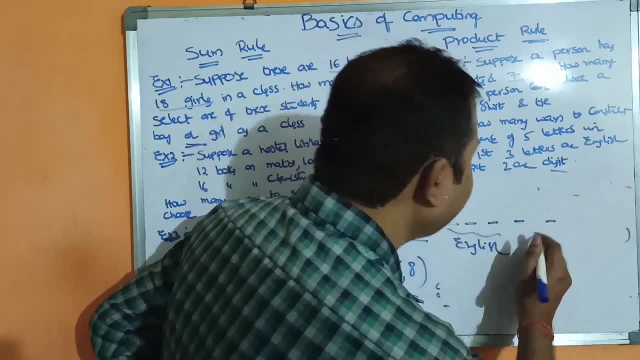 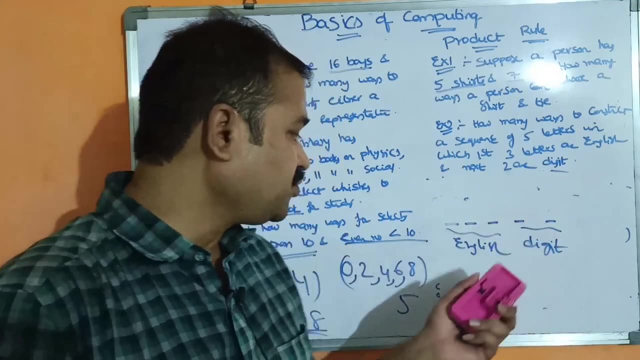 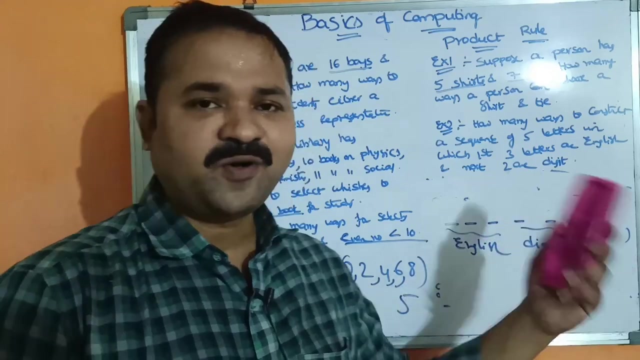 digit and the next two- two are digit, so the next two are digits. so we have to find out how many ways are there in order to select the first three letters as english and the next two as digit? okay, so here we have to perform both the tasks. so task t1 means choosing. 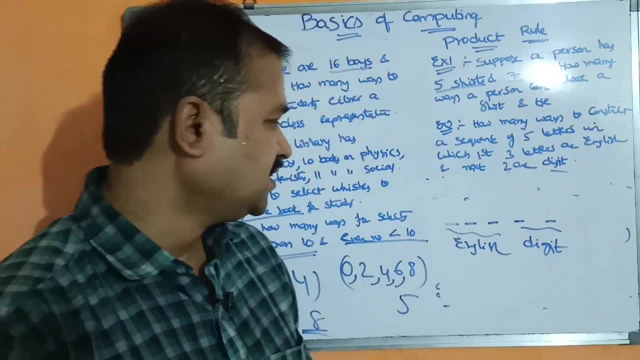 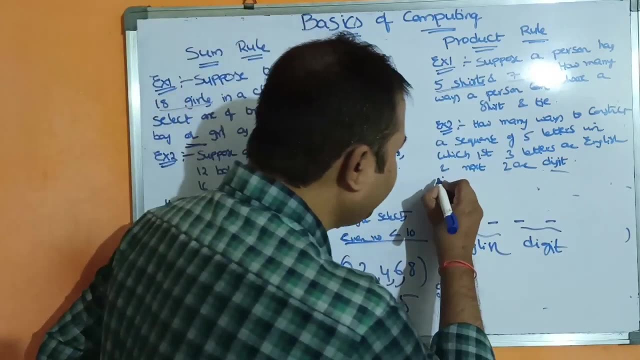 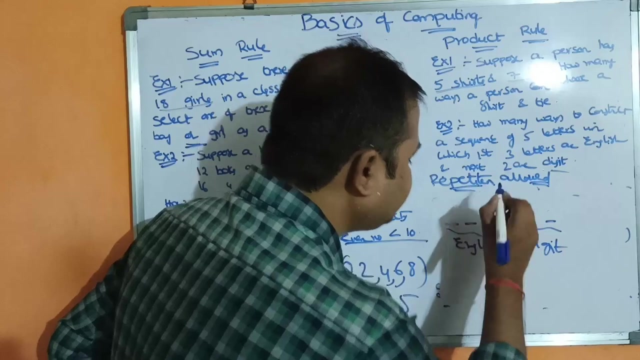 english task t2 means choosing digit. so we have to perform both the tasks, so we have to apply virtual product rule. okay, here we can solve this problem in two ways. the first way is repetition allowed, allowed, and the second way is repetition is not allowed, repetition is not allowed. so here also 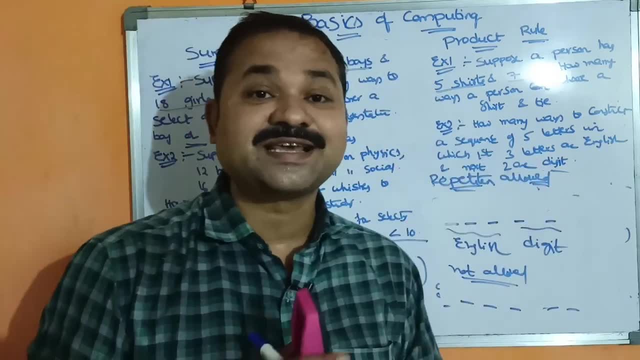 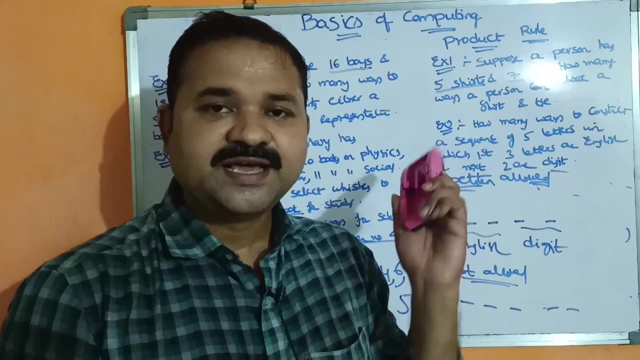 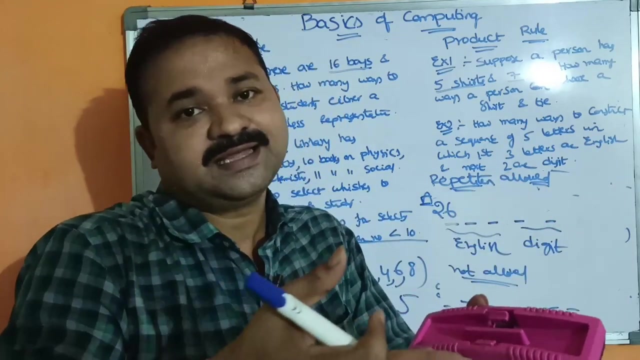 same sequence. so here the repetition is allowed. okay, so in order to select the first letter, we have 26 combinations. are there 26 ways? are there? here repetition is allowed. so that means, if the first letter is a, then the second letter may also a, then the second letter may also contain a. okay, so, 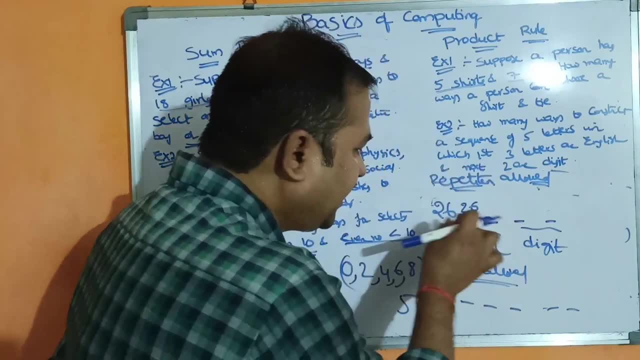 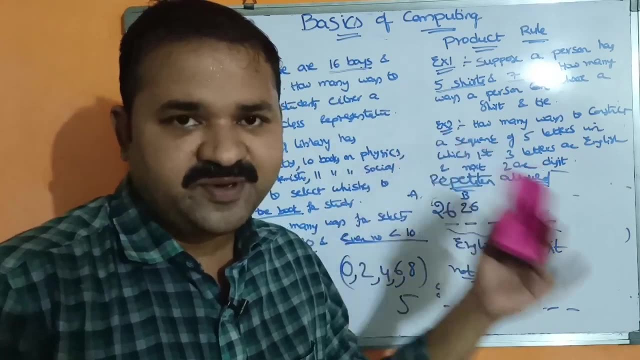 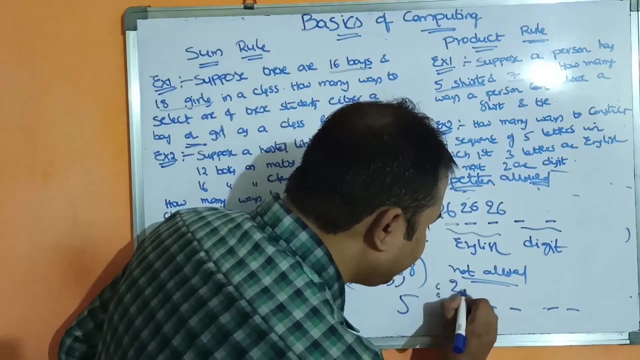 how many letters are there? 26 letters, if the first letter is a, second letter is b, and then the third letter may contains a or b also there is no problem. why? because here the repetition is allowed. okay, so here also 26 combinations. if we consider this one, let the first letter is 26, but here the repetition is not allowed. 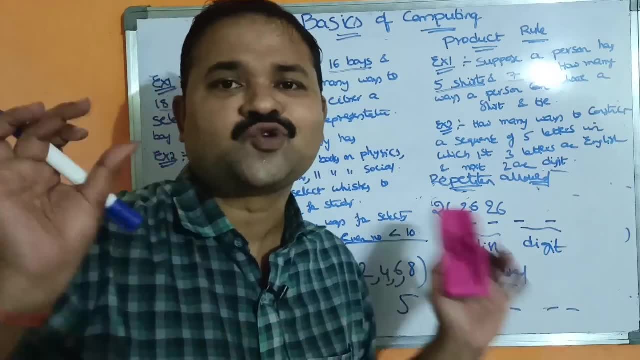 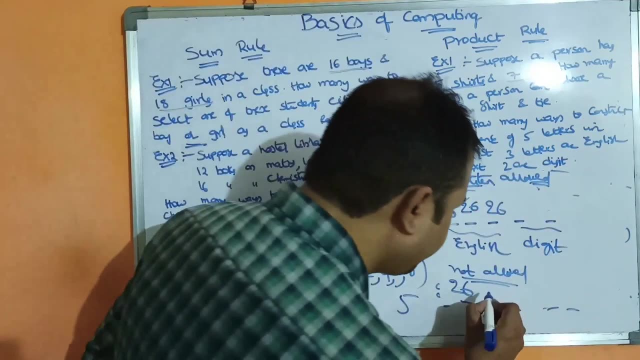 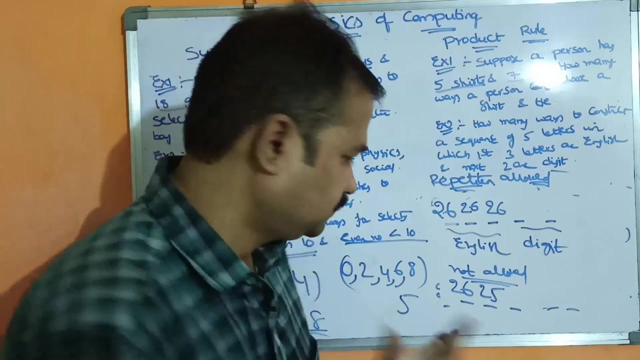 that means if the first letter is a, then the second letter should not be a. so we have to subtract 1 from 26. why? because second letter never be a, so 25, next third letter, never be first letter and second letter. so we have to subtract 2. why? because if the first letter is a, 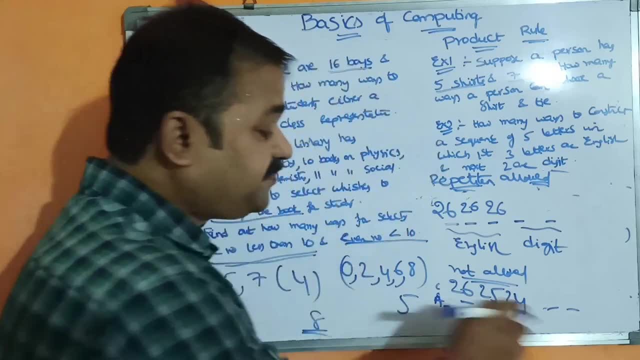 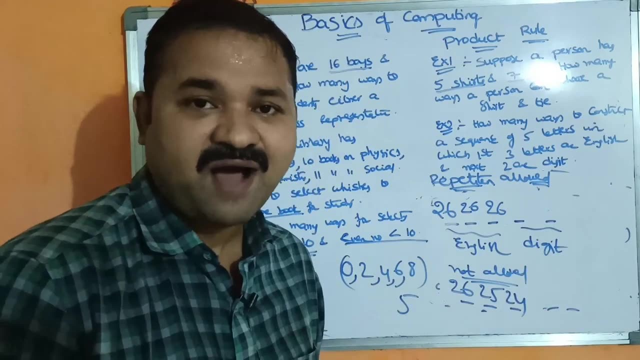 let. the second letter is b, then the third letter can never be a or b, so we have to subtract 2. okay, and let let us consider digit. how many digits are there? we have 10 digits, from 0 to 9, so first contains 10 digits, here the 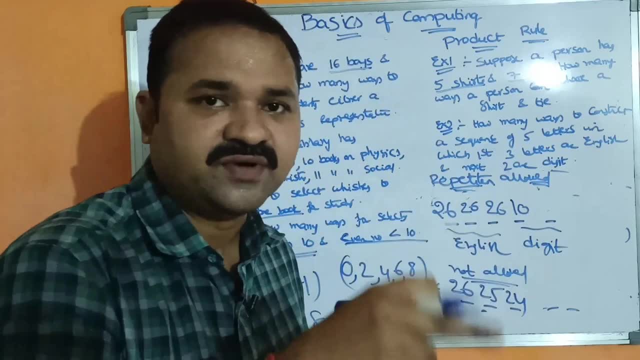 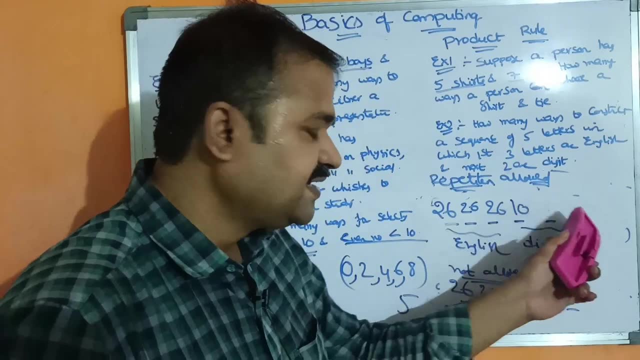 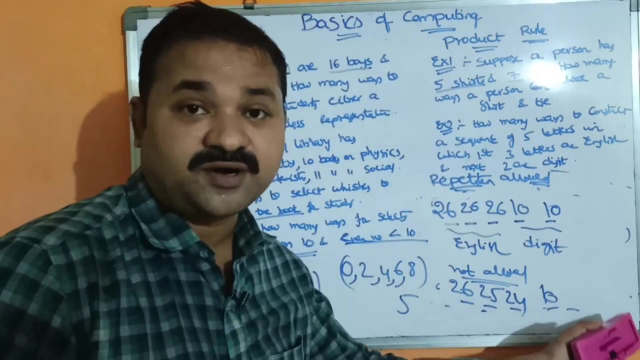 repetition allowed. that means, if the first digit is 5, then the second digit, if the fourth digit is 5. here here we have 2 digits only. if the first digit is 5, then the second digit may be 5 also, so 10 combinations. so here the first one is 10, but here the repetition is not allowed. that means, 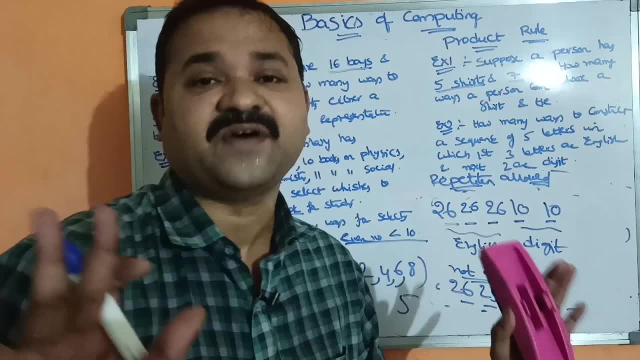 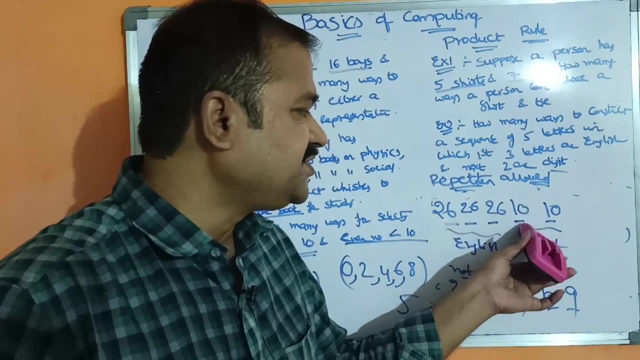 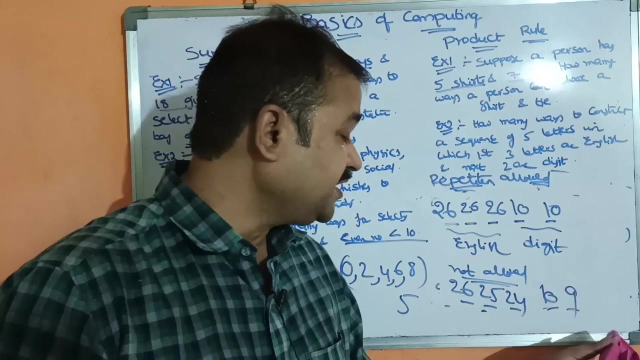 if this is 5, then it can never be okay. so we have 9 digits. perform the multiplication 26 into 26 into 26 into 10 into 10. so this is nothing but the solution for the first one: 26 into 25, into 24, into 10, into 9. this 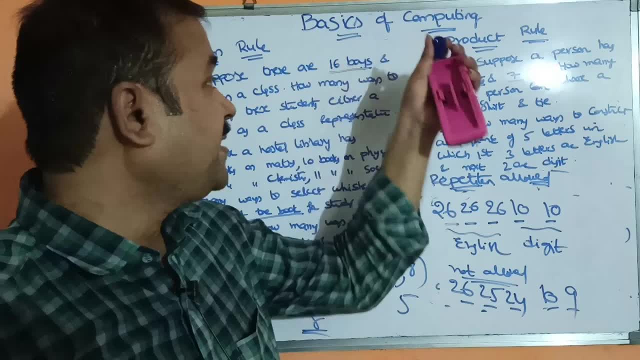 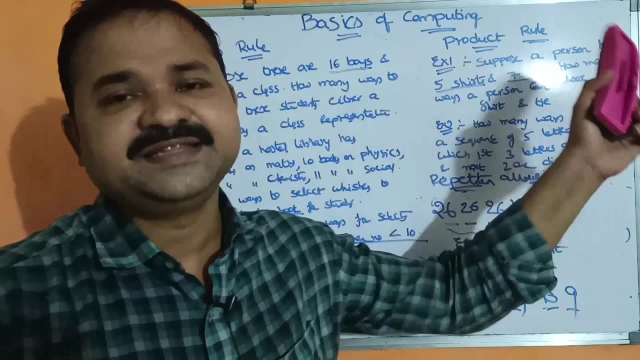 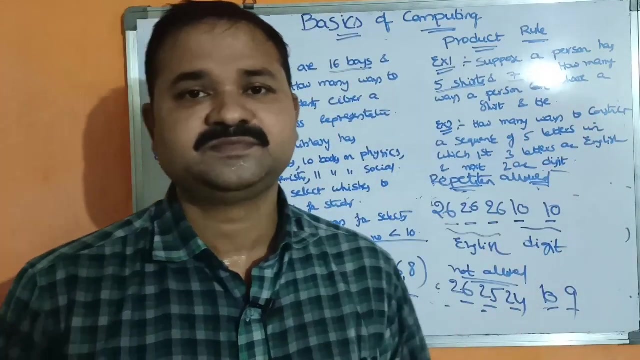 is the solution for the second problem. so this is about basics of computing, sum rule and product rule. so we can solve any problem very, very easily by seeing the problem: either either: or means sum rule, both the tasks means product rule, that's it.